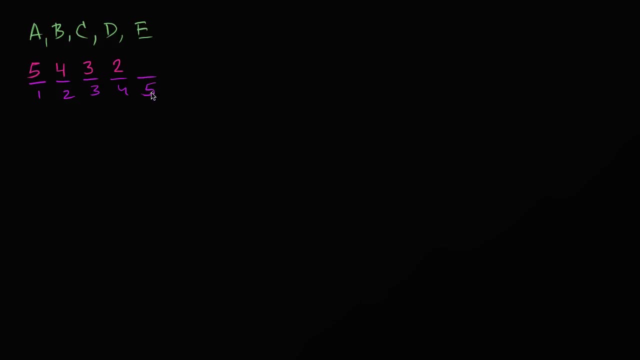 and for each of those, how many possibilities are there for the fifth seat? Well, for each of those scenarios, we only have one person who hasn't sat down left. so there's one possibility, And so the number of permutations, the number of. let me write this down. 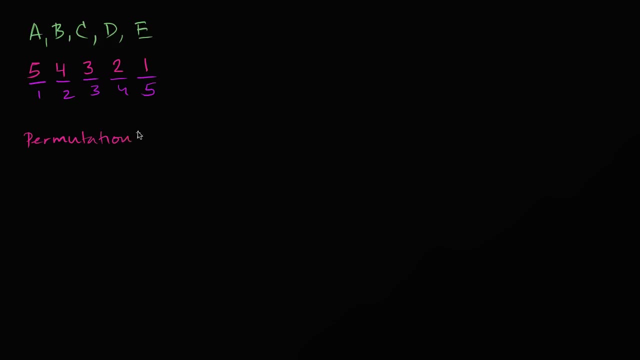 the number of permutations, permutations of seating these five people in five chairs, is five factorial. Five factorial, which is equal to five times four times three times two times one, which of course is equal to- let's see, 20 times six, which is equal to 120.. 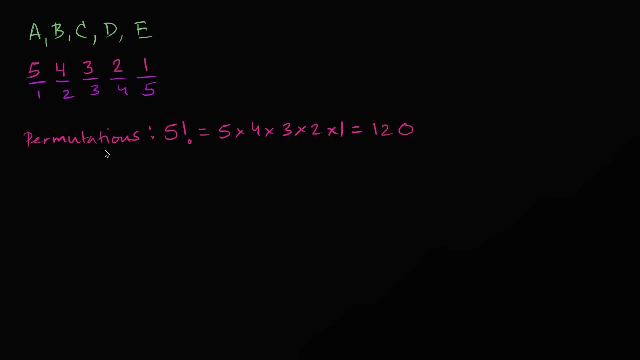 And we've already covered this in a previous video. But now let's do something, maybe more interesting or maybe you might find it less interesting. Let's say that we still have. let's still say we have these five people, but we don't have as many chairs. 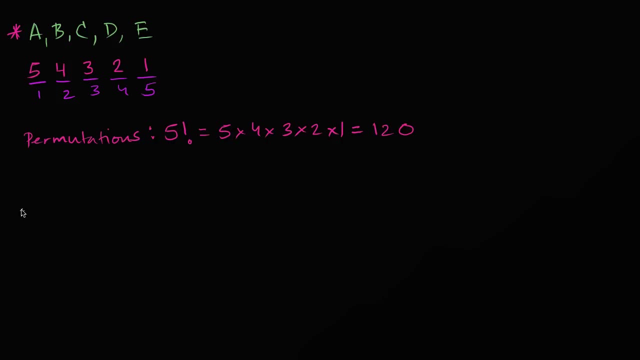 so not everyone is going to be able to sit down. So let's say that we only have three chairs, So we have chair one, we have chair two and we have chair three. So how many ways can you have five people where only three of them are going to sit down? 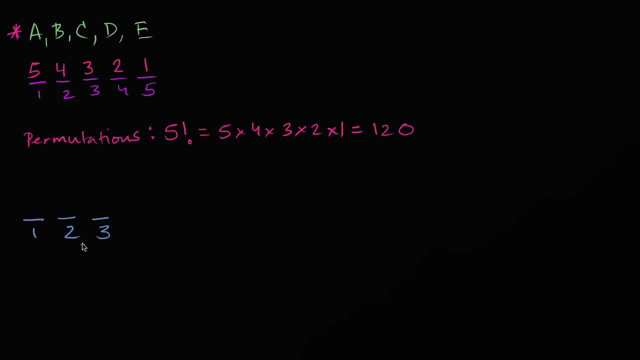 in these three chairs, And we care which chair they sit in, and I encourage you to pause the video and think about it. So I am assuming you have had your go at it, So let's use the same logic. So how many if we seat them in order? 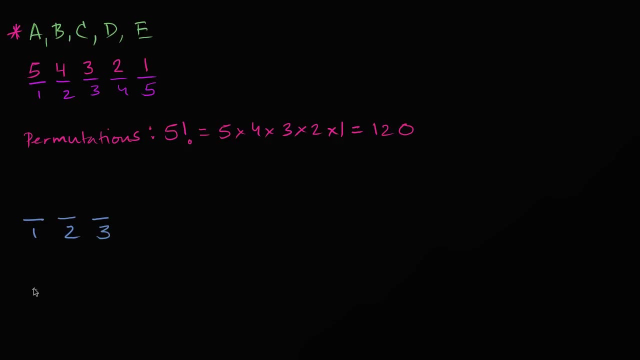 we might as well. how many different people, if we haven't sat anyone yet. how many different people could sit in seat one? Well, we could have. if no one sat down. we have five different people. Well, five different people could sit in seat one. 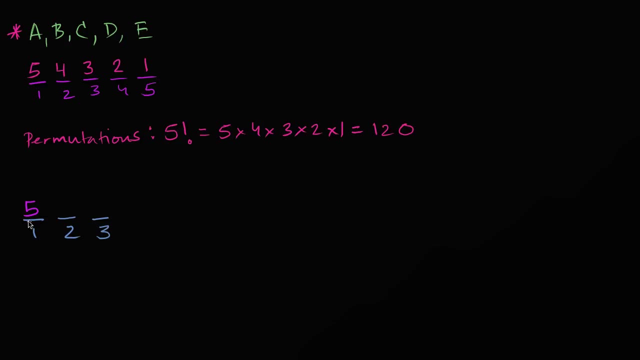 Well, for each of these scenarios where one person has already sat in seat one, how many people could sit in seat two? Well, in each of these scenarios, if one person has sat down, there's four people left who haven't been seated. 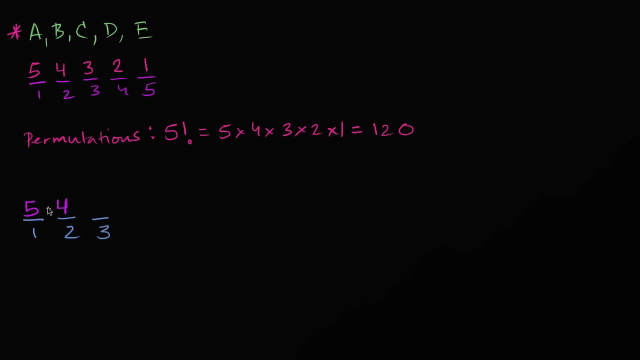 so four people could sit in seat two. So we have five times four scenarios where we have seated seats one and seat two. Now, for each of those 20 scenarios, how many people could sit in seat three? Well, we haven't sat, we haven't. 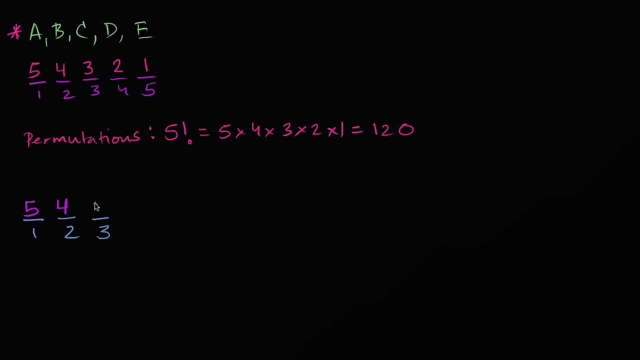 we haven't seaten or sat three of the people yet. So for each of these 20, we could put three different people in seat three. So that gives us five times four times three scenarios. So this is equal to five times four times three scenarios. 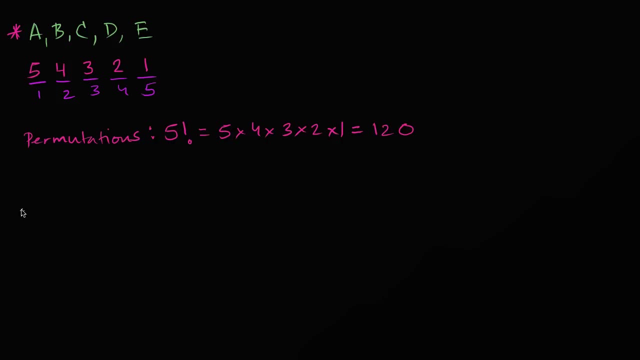 So not everyone is going to be able to sit down. So let's say that we only have three chairs, So we have chair one, we have chair two and we have chair three. So how many ways can you have five people where only three of them are going to sit down? 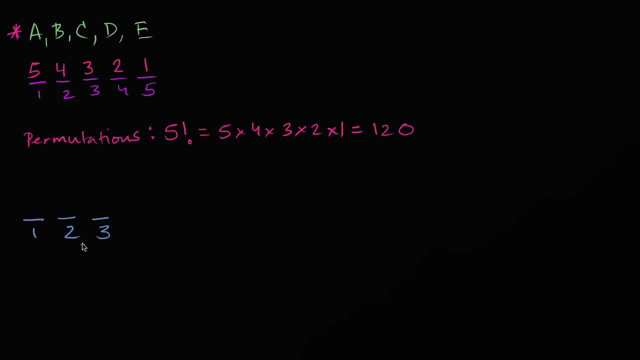 in these three chairs, And we care which chair they sit in, And I encourage you to pause the video and think about it. So I am assuming you have had your go at it, So let's use the same logic. So how many if we seat them in order? 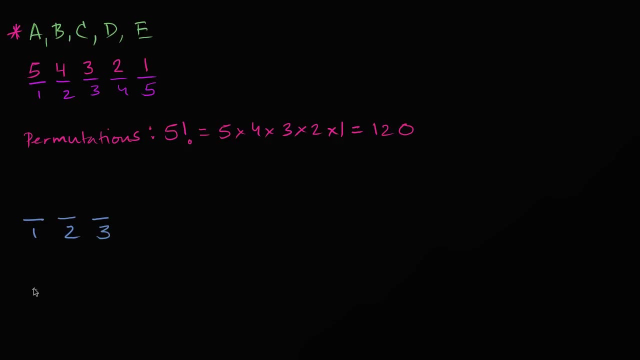 we might as well. how many different people, if we haven't sat anyone yet. how many different people could sit in seat one? Well, we could have. if no one sat down. we have five different people. Well, five different people could sit in seat one. 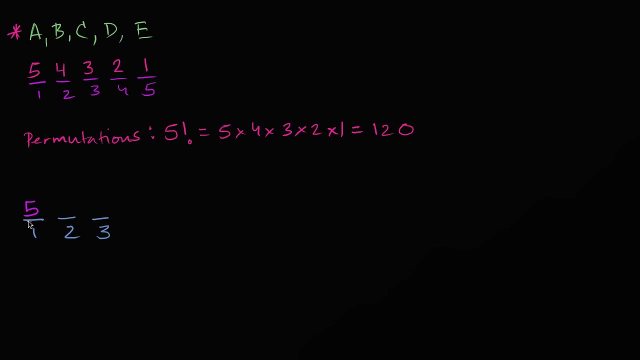 Well, for each of these scenarios where one person has already sat in seat one, how many people could sit in seat two? Well, in each of these scenarios, if one person has sat down, there's four people left who haven't been seated. 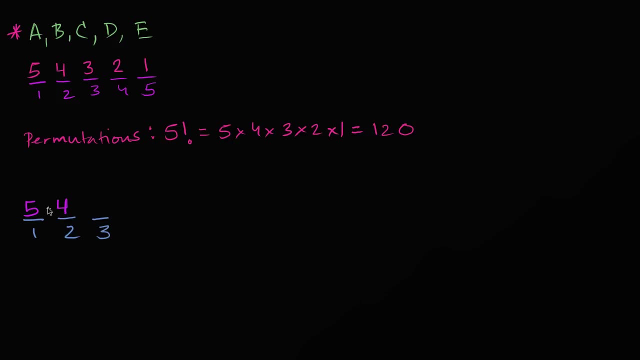 So four people could sit in seat two. So we have five times four scenarios where we have seated seats one and seat two. Now, for each of those 20 scenarios, how many people could sit in seat three? Well, we haven't sat, we haven't. 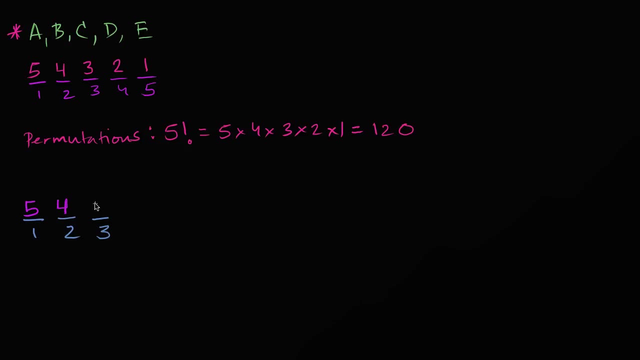 we haven't seaten or sat three of the people yet. So for each of these 20, we could put three different people in seat three. So that gives us five times four times three scenarios. So this is equal to five times four times three scenarios. 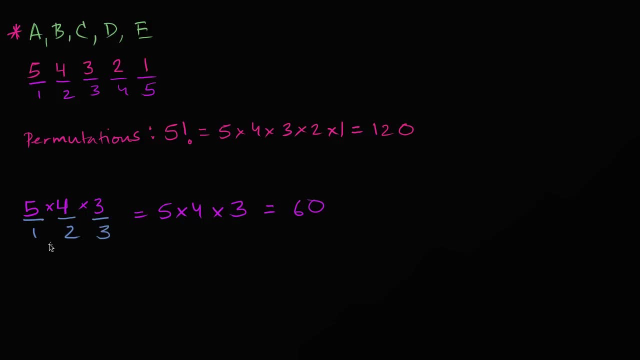 which is equal to this is equal to 60. So there's 60 permutations of sitting five people in three chairs. Now this and this is my brain. you know, whenever I start to think in terms of permutations, I actually 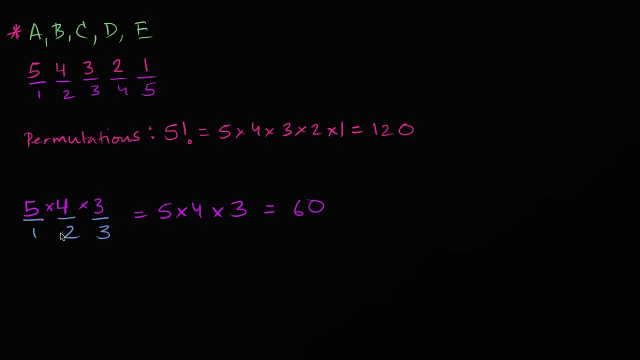 think in these ways. I just literally draw it out because, especially you know, I don't like formulas. I like to actually conceptualize and visualize what I'm doing. But you might say: hey, you know, when we just did five different people. 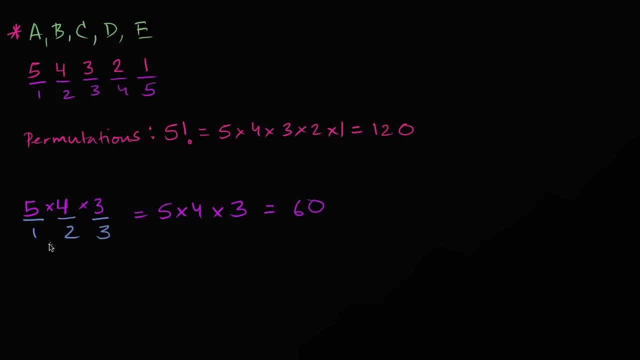 which is equal to this is equal to 60. So there's 60 permutations of sitting five people in three chairs. Now this and this is my brain. you know, whenever I start to think in terms of permutations, I actually think in these ways. 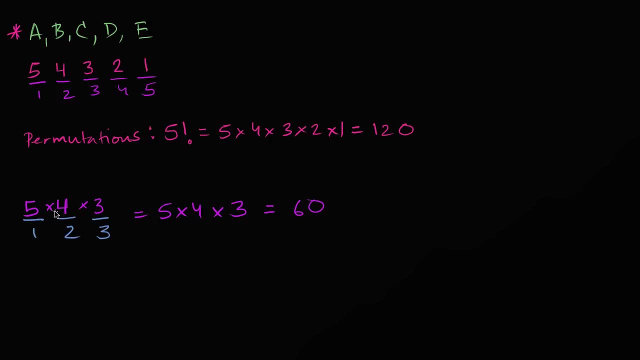 I just literally draw it out because, especially you know, I don't like formulas, I like to actually conceptualize and visualize what I'm doing. But you might say: hey, you know, when we just did five different people in five different chairs, 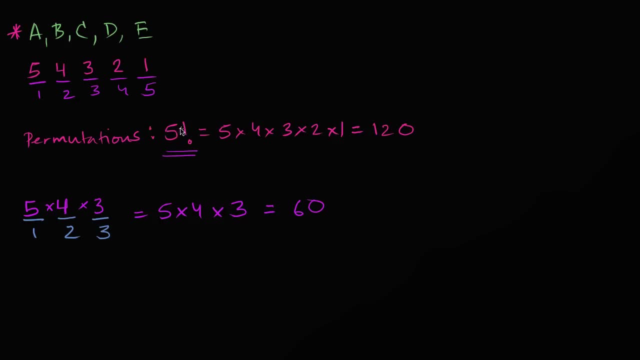 and we cared which seat they sit in. we had this five factorial. but you know, factorial is kind of a neat little operation there. How can I relate factorial to what we did, to what we did just now? Well, it looks like we kind of did factorial. 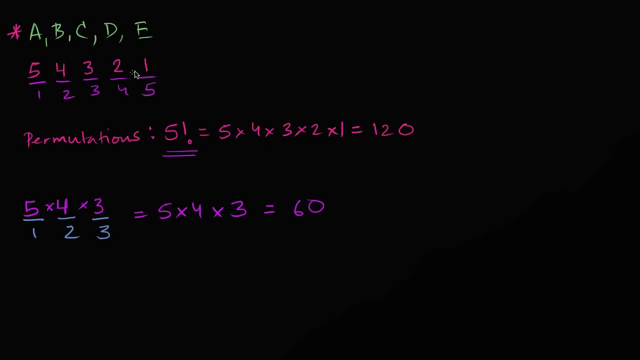 but then we stopped. We stopped at we didn't go times two times one. So one way that we, one way to think about what we just did is we just did. one way to think about what we just did is we just did. 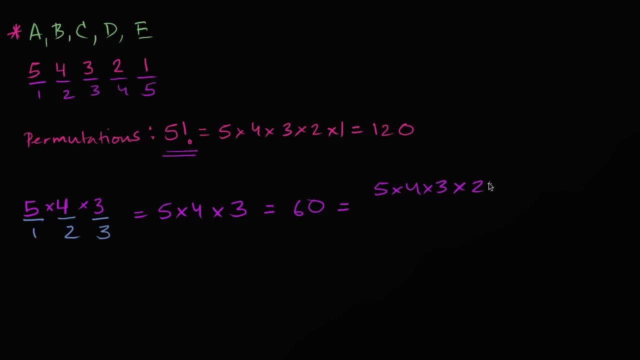 five times four times three times two times one. But of course we actually didn't do the two times one. So you could take that and you could divide by two times one, And if you did that, then this two times one would cancel with that two times one. 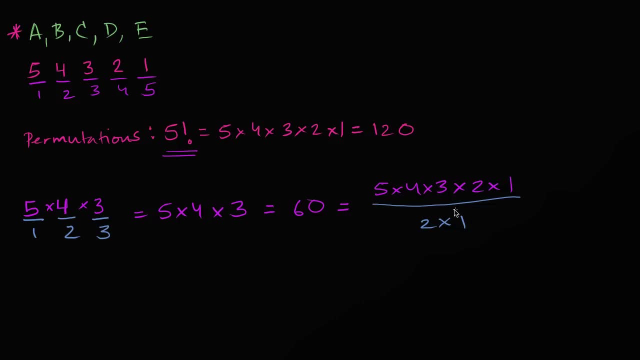 and you'd be left with five times four times three. And the whole reason I'm writing this way is that now I could write it in terms of factorial. I could write this as five factorial, five factorial over two, factorial over two factorial. 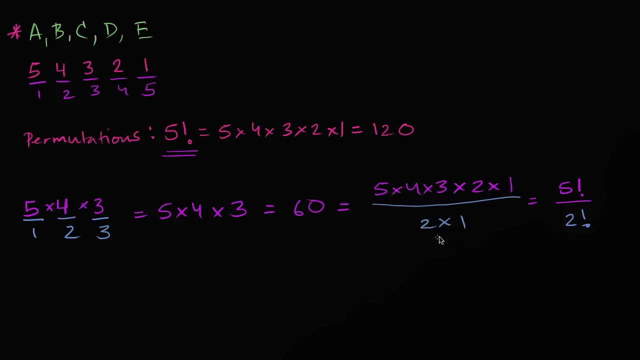 over two factorial. But then you might have the question: well, where did this two come from? Where did you know I have three seats? Where did this two come from? Well, think about it. I multiplied five times, four times three. 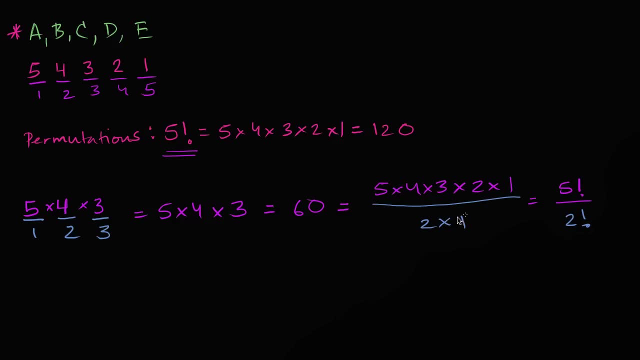 I kept going until I had that many seats and then I didn't do the remainder. So the number of, so the things that I left out, the things that I left out, that was essentially the number of people minus the number of chairs. 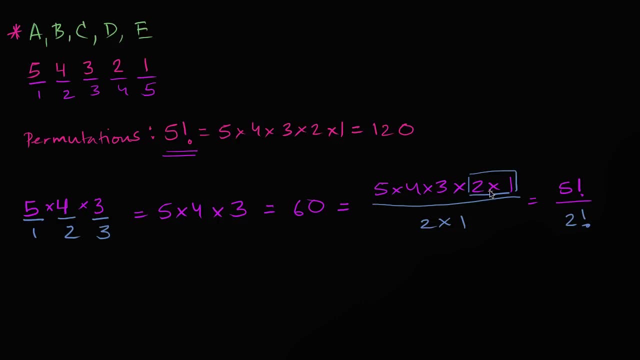 So I was trying to put five things in three places, So five minus three. that gave me two left over, So I could write it like this: I could write it as five- let me use those same colors. I could write it as five- factorial. 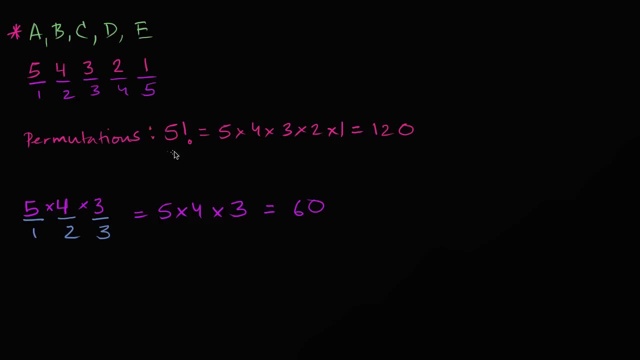 in five different chairs and we cared which seat they sit in. we had this five factorial. You know, factorial is kind of a neat little operation there. How can I relate factorial to what we did, to what we did just now? Well, it looks like we kind of did factorial. 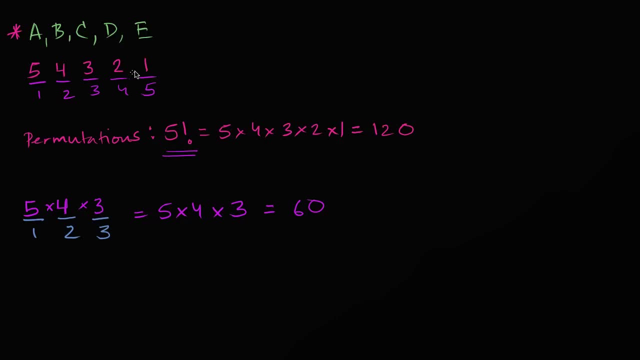 but then we stopped. We stopped at. we didn't go times two times one. We stopped at. we didn't go times two times one. We stopped at. we didn't go times two times one. So one way that we, one way to think about: 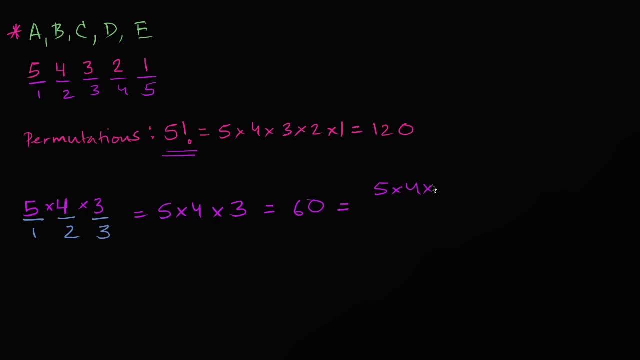 what we just did is we just did five times four times three times two times one, But of course we actually didn't do the two times one. So you could take that and you could divide by two times one, And if you did that, then this two times one. 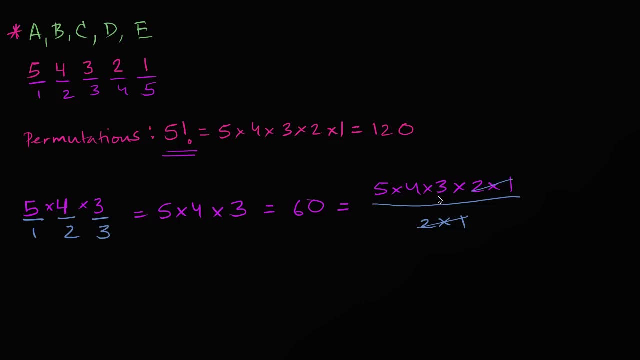 would cancel with that two times one and you'd be left with five times four times three. And the whole reason I'm writing this way is that now I could write it in terms of factorial, I could write this as five factorial over two, factorial over two factorial. 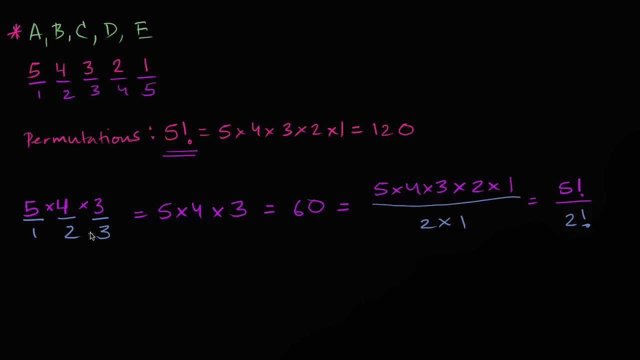 But then you might have the question: well, where did this two come from? Where did you know I have three seats? Where did this two come from? Well, think about it. I multiplied five times four times three. I kept going until I had that many seats. 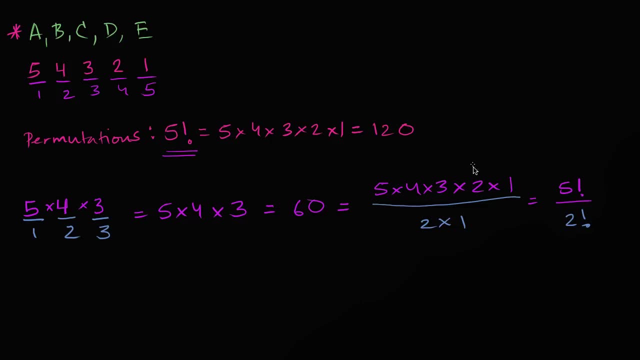 and then I didn't do the remainder. So the number of, so the things that I left out, the things that I left out, that was essentially the number of people minus the number of chairs. So I was trying to put five things in three places. 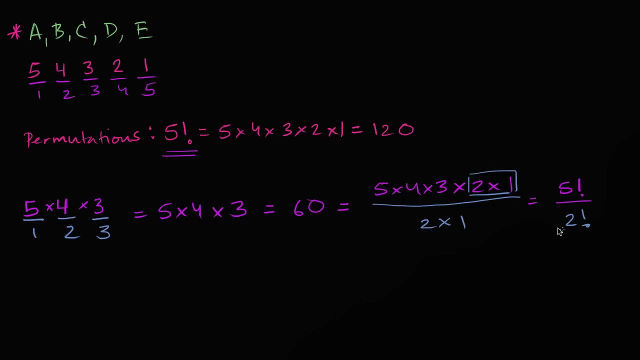 So five minus three. that gave me two left over. So I could write it like this: I could write it as five- let me use those same colors. I could write it as five- factorial- over over five minus three, which of course is two, five minus three factorial. 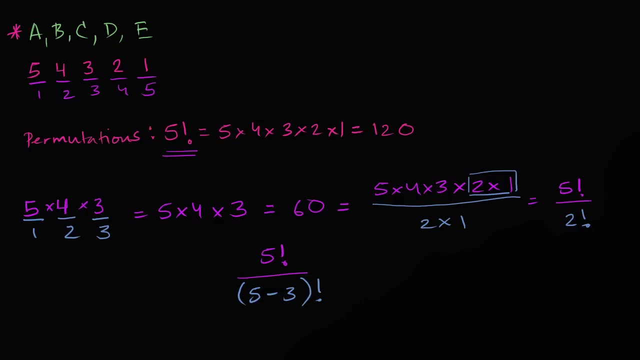 And so another way of thinking about it, if we wanted to generalize is: if you're trying to put, if you're trying to figure out the number of permutations- and there's a bunch of notations for writing this- if you're trying to figure out the number of permutations, 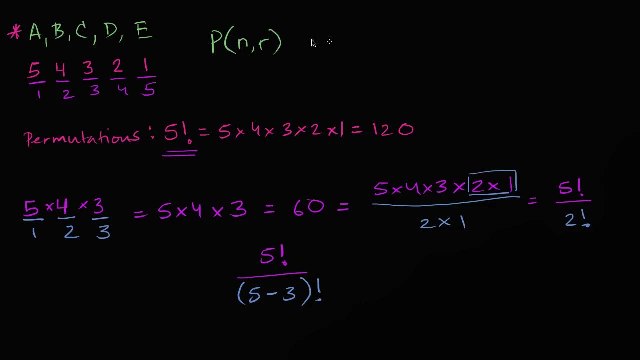 where you could put n people in r seats, or the number of permutations you could put n people in r seats, and there's other notations as well. well, this is just going to be n factorial over n minus r factorial. Here n was five. 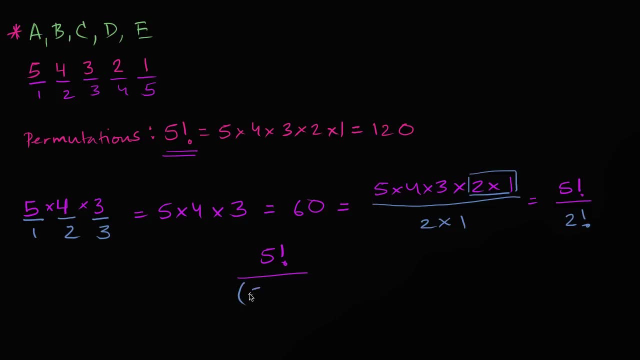 over over five minus three, which of course is two five minus three factorial. And so another way of thinking about it, if we wanted to generalize, is if you're trying to put, if you're trying to figure out the number of permutations. 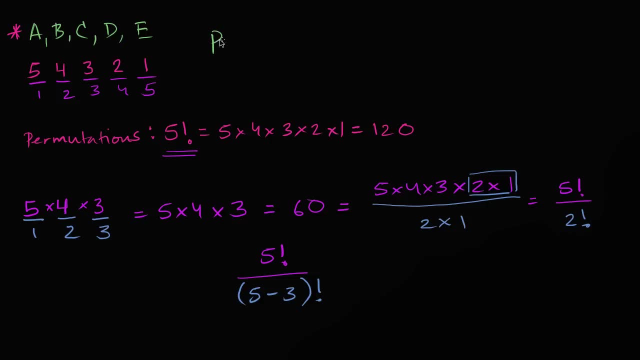 and there's a bunch of notations for writing this. If you're trying to figure out the number of permutations where you could put n people in r seats, or the number of permutations you could put n people in r seats- and there's other notations as well- 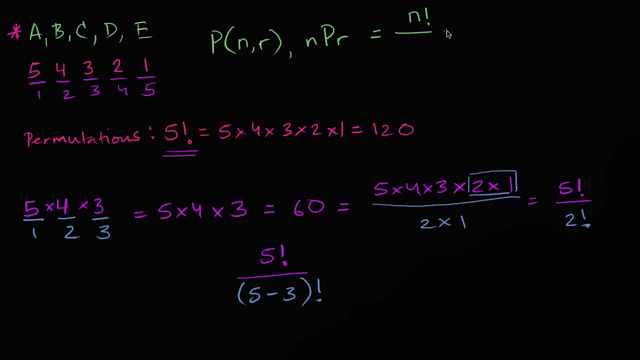 Well, this is just going to be n factorial over n minus r factorial. Here n was five, r was three and minus five minus three is two. Now you'll see this in a probability or statistics class and you know people might memorize this thing. 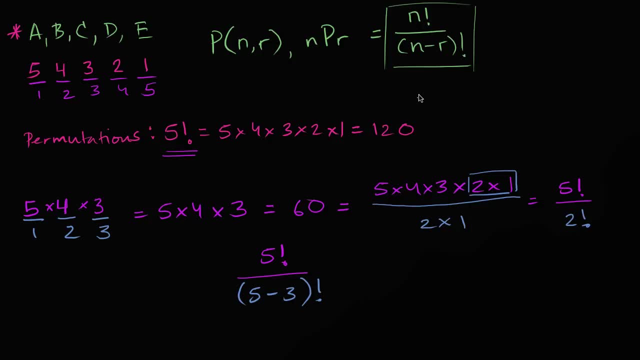 and it seems like this kind of daunting thing. I'll just tell you right now: the whole reason why I just showed this to you is so that you could connect it with what you might see in your textbook or what you might see in a class. 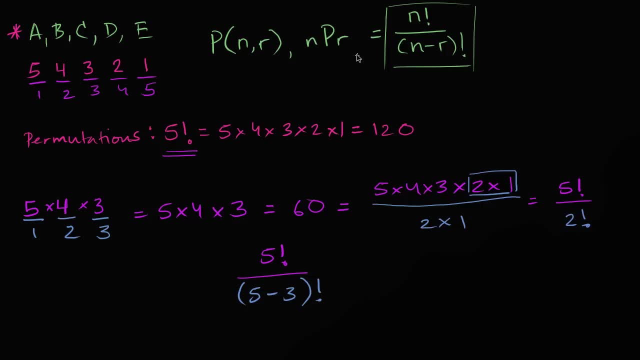 or when you see this type of formula, you see that it's not, you know, coming out of you know, it's not some type of voodoo magic. but I will tell you that for me personally, I never use this formula. 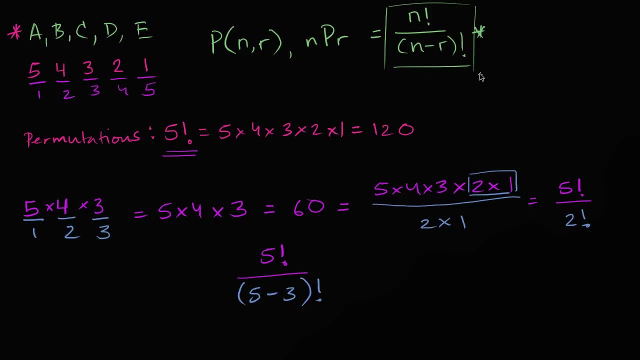 I always reason it through, because if you just memorize the formula you're always like: wait, does this formula apply there? What's n, What's r? But if you reason it through it comes out of straight logic. You don't have to memorize anything. 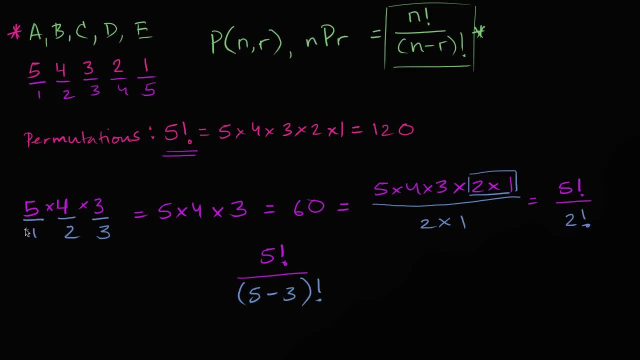 You don't feel like you're just memorizing without understanding. You're just using your deductive reasoning, your logic, and that's especially valuable because, as we'll see, not every scenario is going to fit so cleanly into what we did. 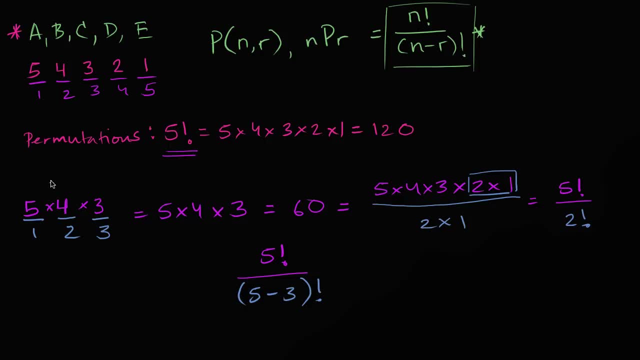 There might be some tweaks on this where, like you know, maybe only person B likes sitting in one of the chairs, or who knows what it might be, and then your formula is going to be useless. So I like reasoning through it like this: 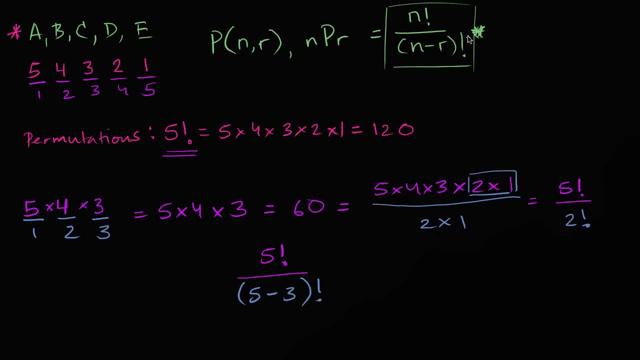 but I just showed you this so that you could connect it to a formula that you might see in a lecture or in a class.